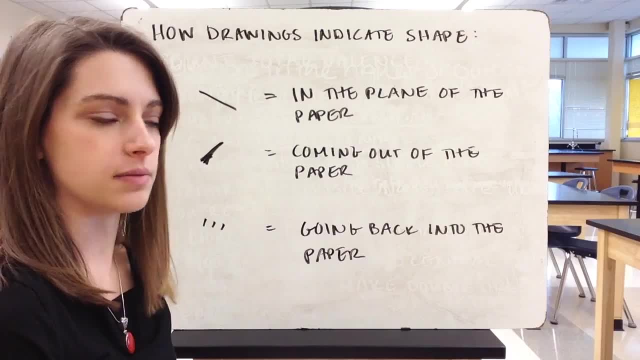 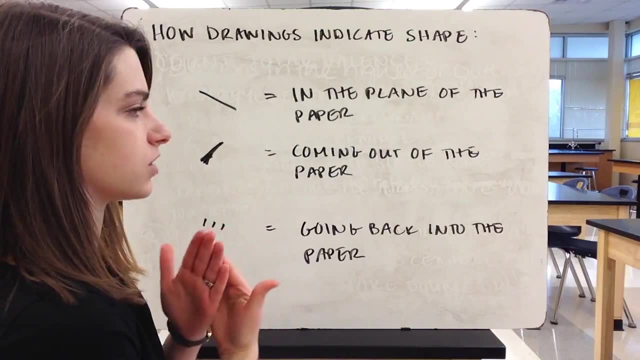 If you draw it as a wedge, that means it's coming out of the paper. So if you're holding your molecule up, that atom is going to be coming towards you. And if you draw a dotted line, that means it's going back into the plane of the paper. 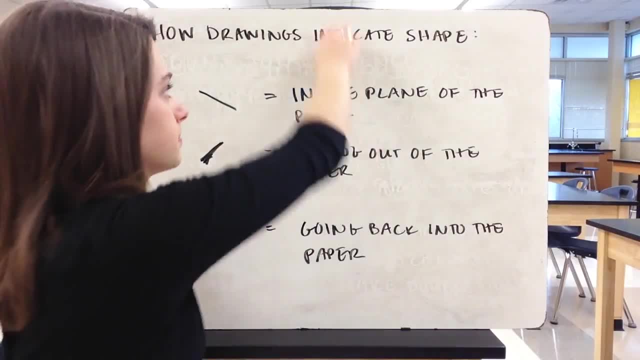 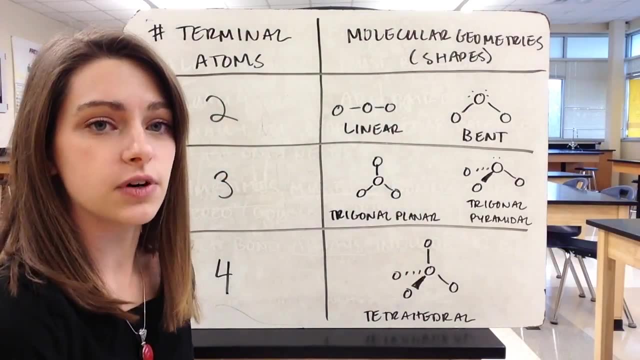 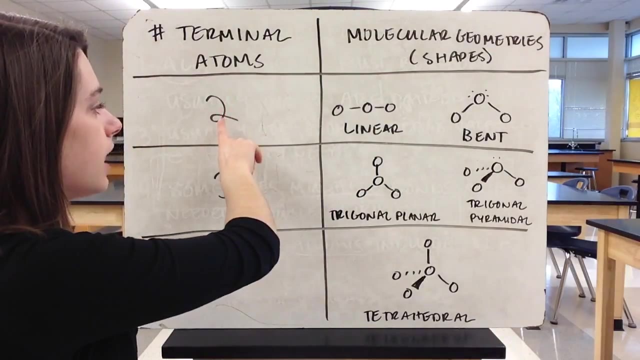 so it's going away from you. We're going to look at examples of all of these. So we're going to focus on five different shapes and they have different shapes depending on how many atoms are around their central atom. So if you have two terminal atoms, 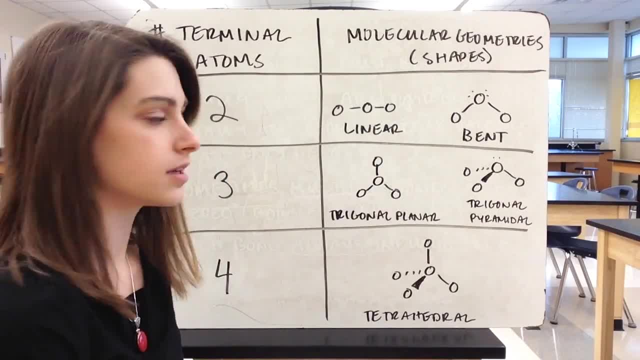 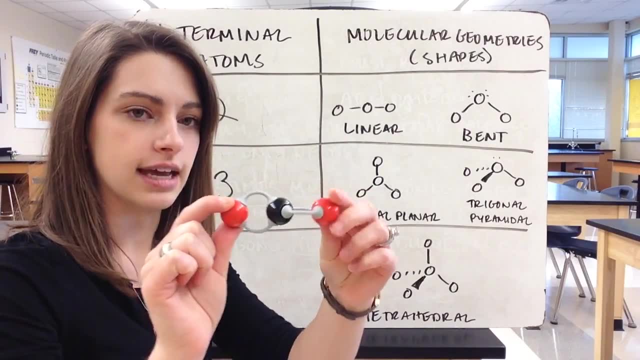 or two atoms around your central atom. you're going to have two possible shapes. Your first shape is linear and that looks something like this. So this is carbon dioxide, CO2.. And if you see, my atoms are in a straight line. 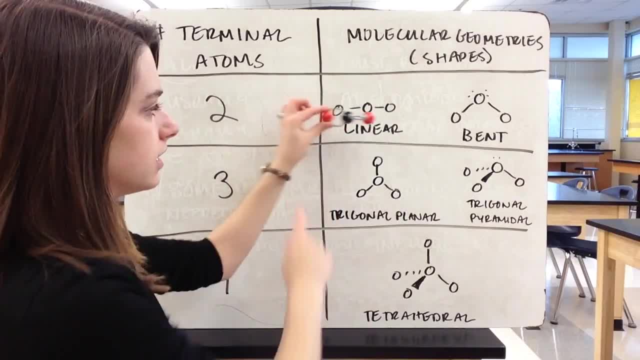 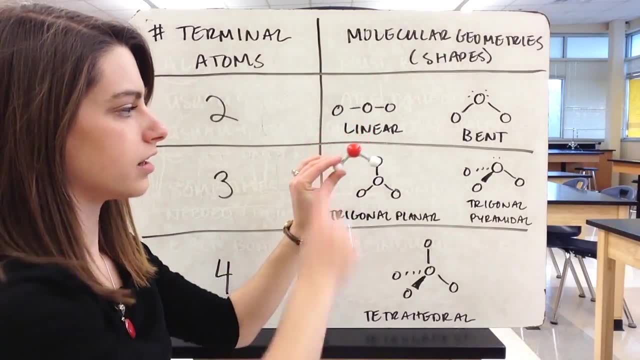 If I were to hold them up against the board. they're all in the same plane, So this is a linear structure. An example of a bentonite structure is water. So water has two electron pairs that appear on the oxygen. They're not in my little model guy. 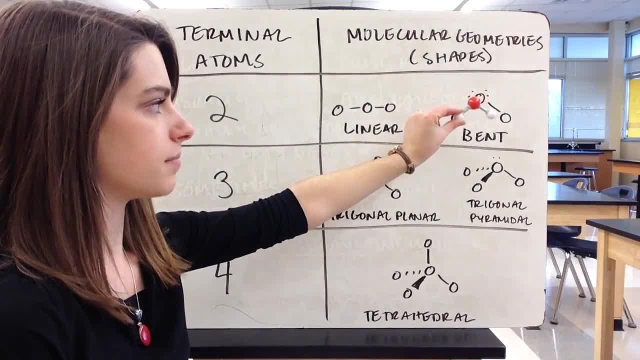 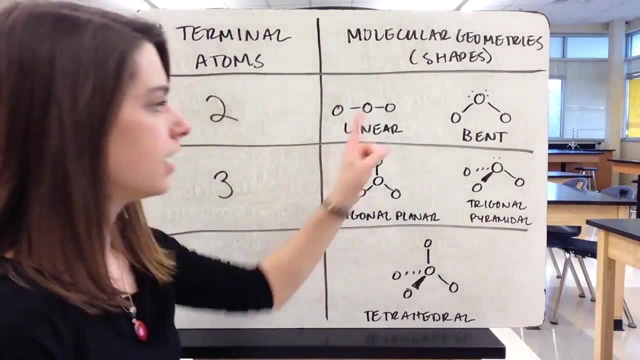 But you can see it bends so that those electron pairs push away on those bonds And this is called bent. That makes sense. The atom is bent. So we have linear and we have bent for our molecules that have two terminal atoms. If we have three terminal atoms, 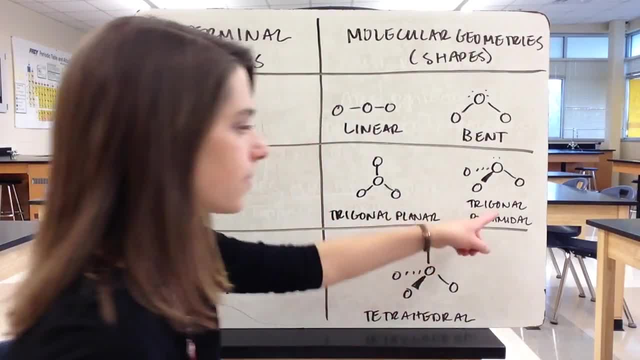 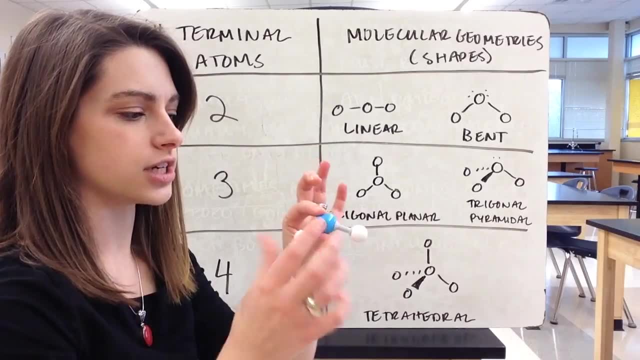 we again have two different options Now. the trigonal pyramidal is the only one I have an example of. So this would be NH3.. So we have our nitrogen. in the middle We have our three hydrogens. If you notice, it's in a slightly 3D shape. 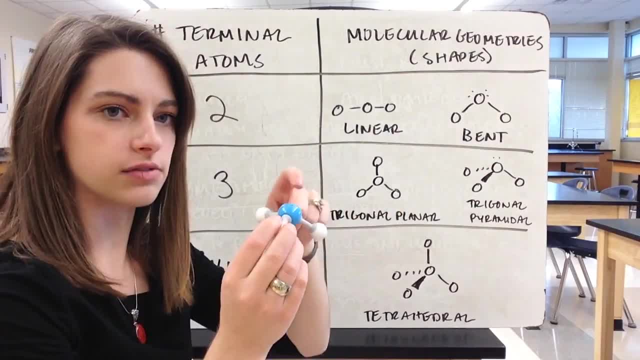 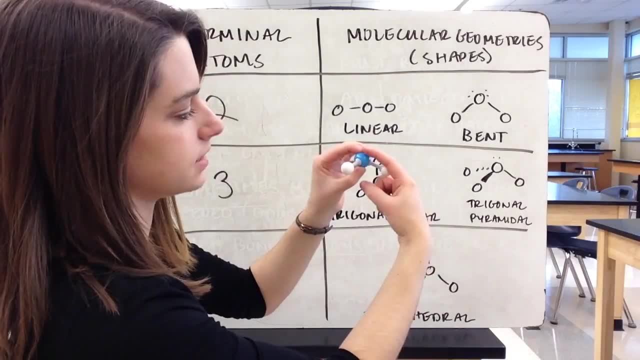 All of these guys are bent slightly away. There would be a lone pair of electrons up here pushing away on our other bonds. So when we draw this we can imagine this bond is in the plane of the paper. This one up here is coming out towards me. 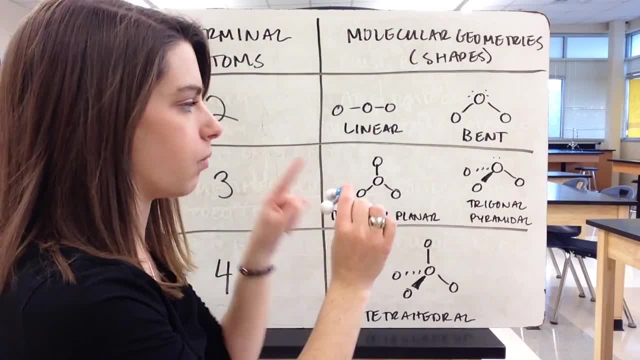 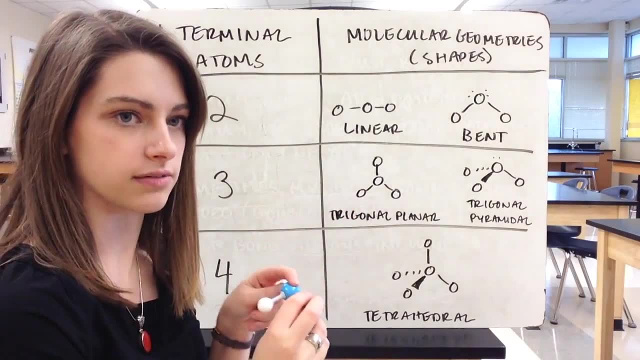 so it's drawn with a wedge, And this one back here is going away from me, so we draw it with a dotted line. The other option for three terminal atoms is if you don't have a lone pair of electrons. That would be like BH3. 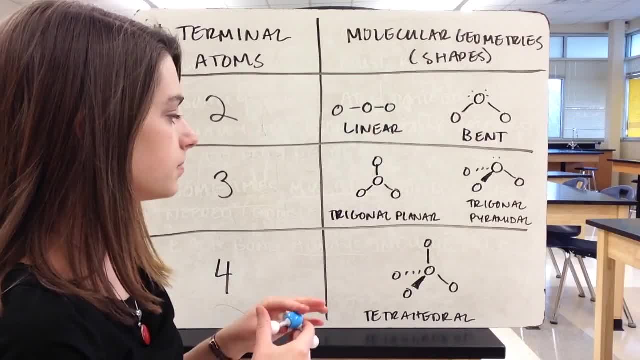 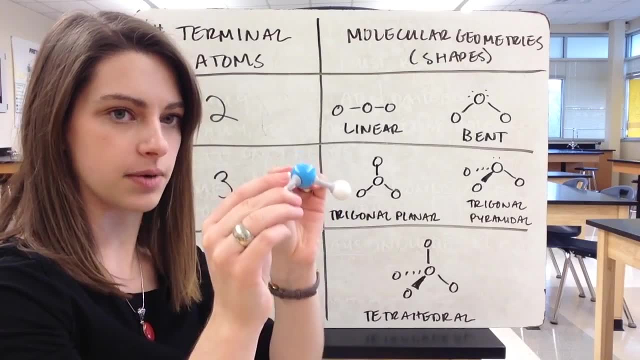 Boron doesn't need all eight, It doesn't need an octet. It would be trigonal planar, So it would be the same shape, except flat. instead of sitting up on its three little legs, It would just be flat.